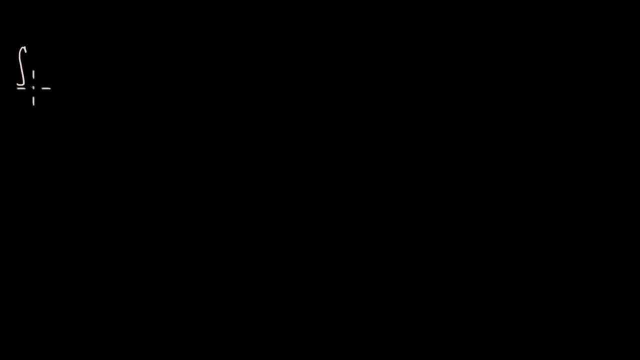 What we're gonna do in this video is try to evaluate the definite integral from zero to pi, of x, cosine of x, dx. Like always, pause this video and see if you can evaluate it yourself. Well, when you immediately look at this, it's not obvious how you just straight up. 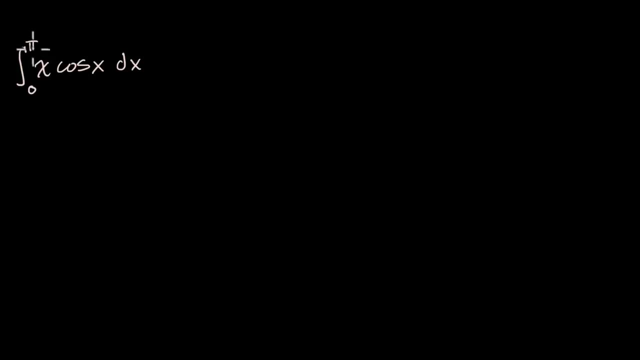 take the antiderivative here and then evaluate that at pi and then subtract from that and evaluate it at zero. So we're probably going to have to use a slightly more sophisticated technique And in general, if you see a product of functions right over here, 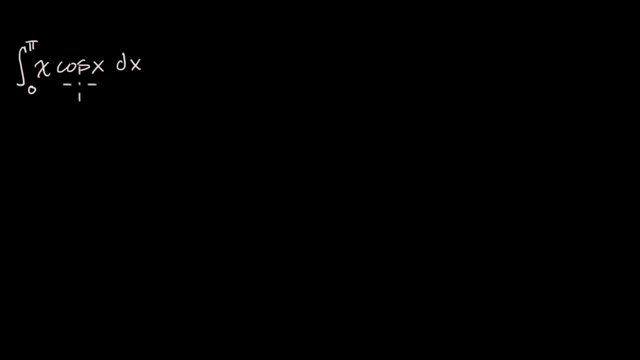 and if one of these functions is fairly straightforward to take the antiderivative of without making it more complicated, like cosine of x and another of the functions like x, if you were to take its derivative it gets simpler. In this case it would just become one. 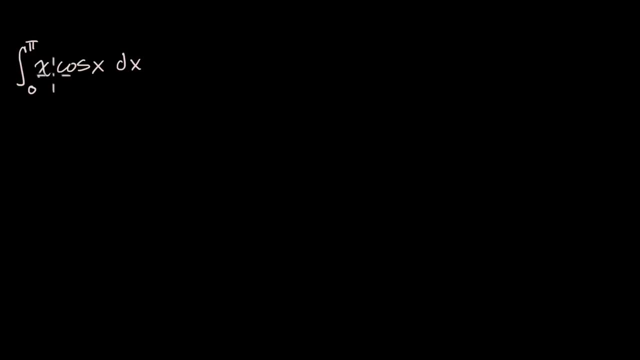 It's a pretty good sign that we should be using integration by parts. So let's just remind ourselves about integration by parts. So, integration by parts. I'll do it right over here, If I have the integral, and I'll just write this. 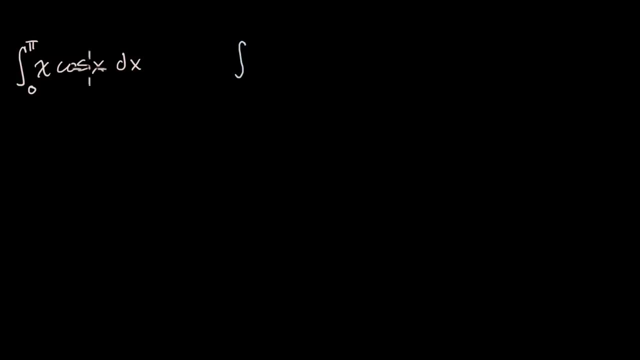 as an indefinite integral. but here we want to take the indefinite integral and then evaluate it at pi and evaluate it at zero. So if I have f of x times g, prime of x, dx, this is going to be equal to- and in other videos we prove this- 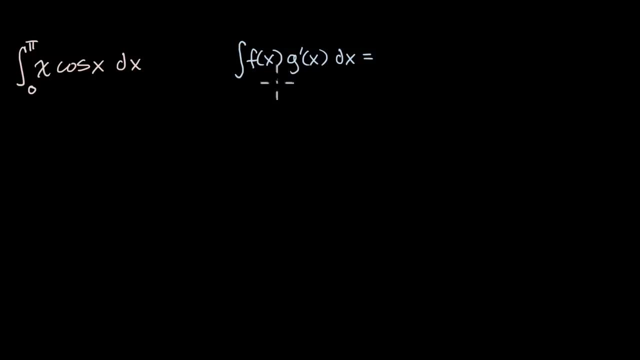 It really just comes straight out of the product rule that you learned in differential calculus. this is going to be equal to f of x times g of x minus. you then swap these around: minus f, prime of x, g of x, dx. And just to reiterate what I said before, 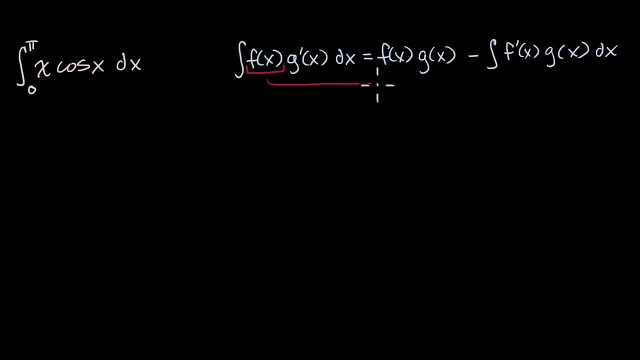 you want to find an f of x that when I take its derivative, it simplifies, it, So simplify. And you want to find a g prime of x that when I take its antiderivative, so when I take its antiderivative. 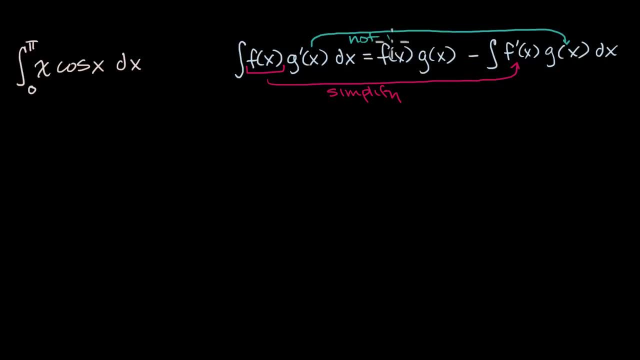 it doesn't get more complicated. So not more complicated, Because if the f of x gets simplified when I take its derivative and the g prime of x does not get more complicated when I take its antiderivative, then this expression will maybe be easier. 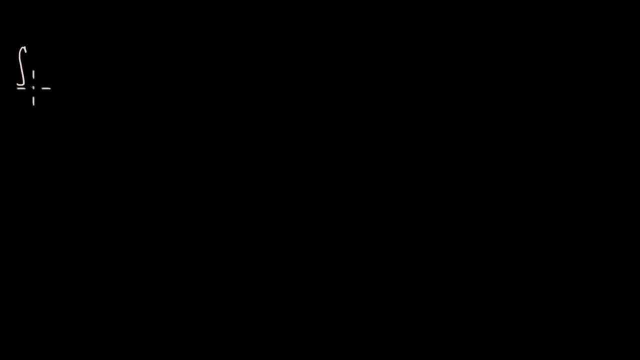 What we're gonna do in this video is try to evaluate the definite integral from zero to pi, of x, cosine of x, dx. Like always, pause this video and see if you can evaluate it yourself. Well, when you immediately look at this, it's not obvious how you just straight up. 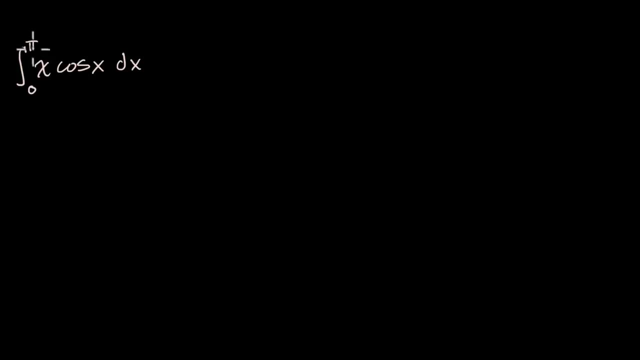 take the antiderivative here and then evaluate that at pi and then subtract from that and evaluate it at zero. So we're probably going to have to use a slightly more sophisticated technique And in general, if you see a product of functions right over here, 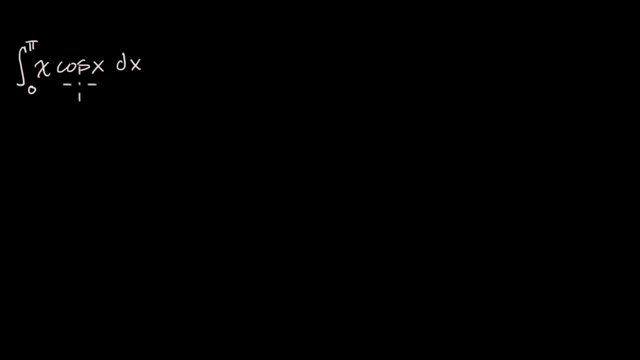 and if one of these functions is fairly straightforward to take the antiderivative of without making it more complicated, like cosine of x and another of the functions like x, if you were to take its derivative it gets simpler. In this case it would just become one. 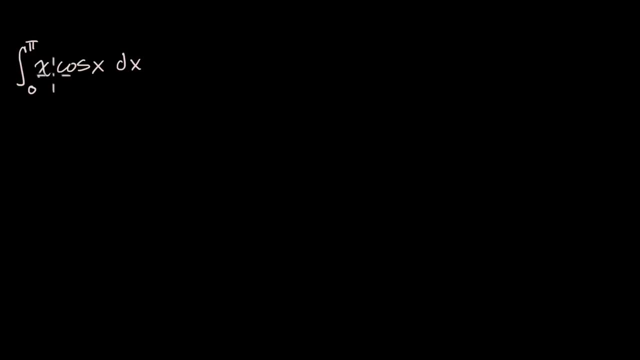 It's a pretty good sign that we should be using integration by parts. So let's just remind ourselves about integration by parts. So, integration by parts. I'll do it right over here, If I have the integral, and I'll just write this. 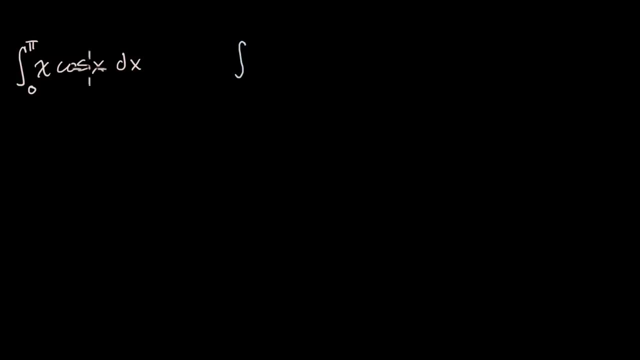 as an indefinite integral. but here we want to take the indefinite integral and then evaluate it at pi and evaluate it at zero. So if I have f of x times g, prime of x, dx, this is going to be equal to- and in other videos we prove this- 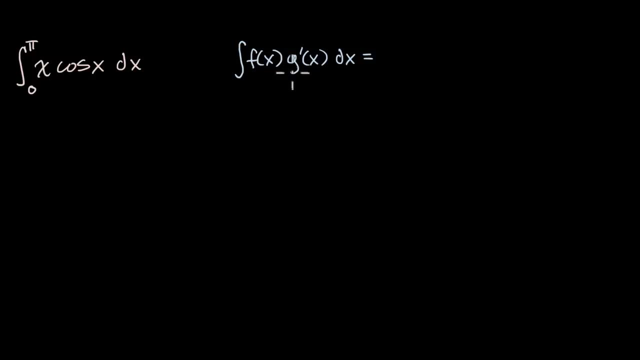 It really just comes straight out of the product rule that you learned in differential calculus. This is going to be equal to f of x times g, prime of x dx. This is going to be equal to f of x times g of x minus. you then swap these around. 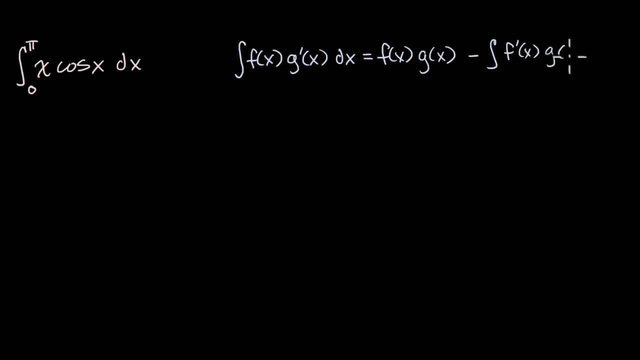 minus f prime of x, g of x, dx. And just to reiterate what I said before, you want to find an f of x that, when I take its derivative, it simplifies it, So simplify. And you want to find a g prime of x. 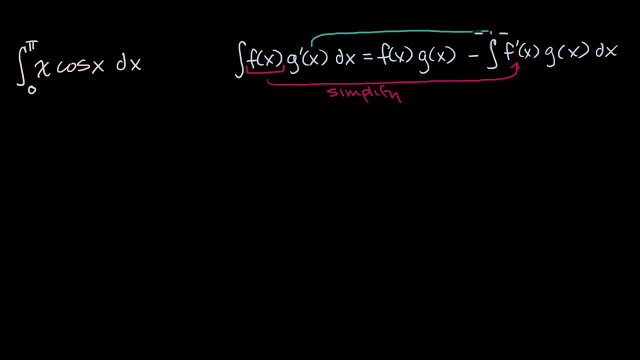 that when I take its antiderivative, so when I take its antiderivative it doesn't get more complicated. So not more complicated, Because if the f of x gets simplified when I take its derivative and the g prime of x does not get more complicated, 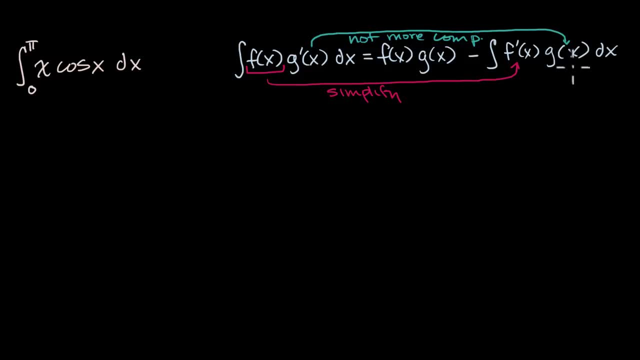 when I take its antiderivative, then this expression will maybe be easier to find: the antiderivative of. So let's do that over here, Between x and cosine of x, which one gets more simple when I take its derivative. Well, the derivative of x is just one. 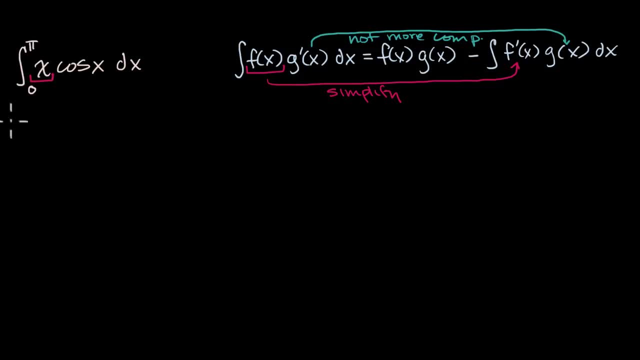 So I'm gonna make that my f of x, So I could write that over here. So my f of x, I will say, is x, in which case f prime of x, f prime of x, is going to be equal to one. And then what would my g prime of x be? 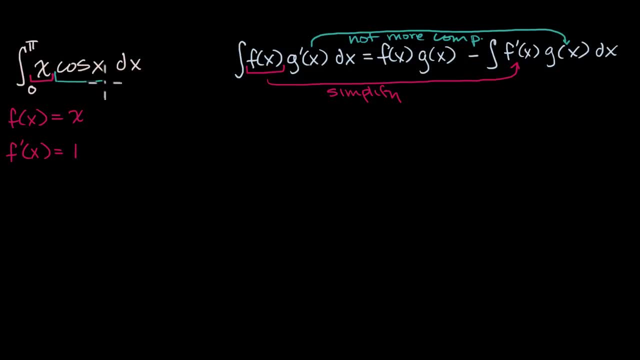 Well, my g prime of x, cosine of x. if I take its antiderivative, it doesn't get more complicated. The antiderivative of cosine of x is sine of x. So let me make that my g prime of x. So g prime of x is equal to cosine of x. 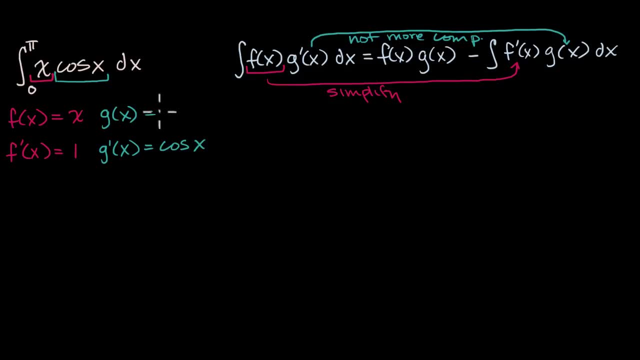 in which case g of x, the antiderivative of cosine of x, well, it's just sine of x, or the other way to think about it, the derivative of sine of x is cosine of x. Now you could think about plus c's and all of that. 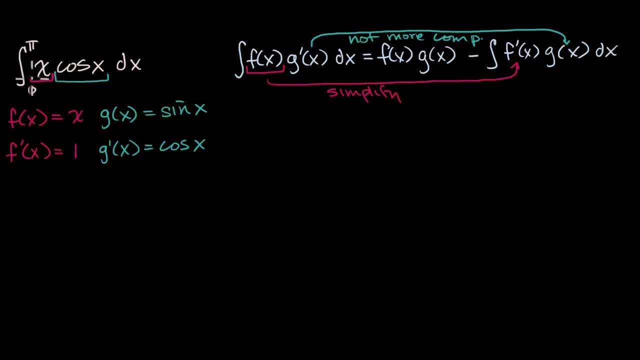 but remember, this is going to be a definite integral, so all those arbitrary constants are going to get canceled out. So now let's think through this. Let's just apply the integration by parts here. In this particular case, all of this is going to be equal to: 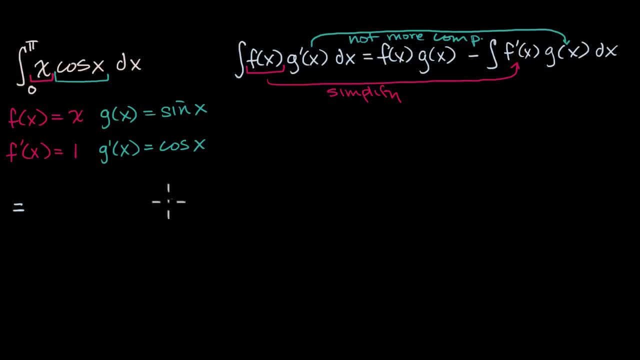 so I'm saying that is equal to this. I'm gonna skip down here. It's going to be equal to f of x times g of x. So that is f of x is x, g of x is sine of x. f of x times g of x. 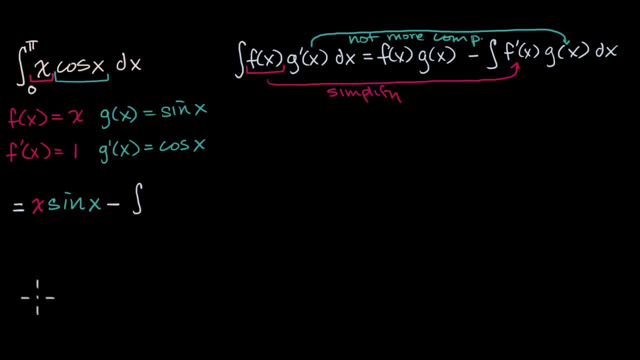 minus the integral of f prime of x. f prime of x is just one. We could write it like that: One times g of x. g of x is sine of x. So we could write it like this: but one times sine of x. 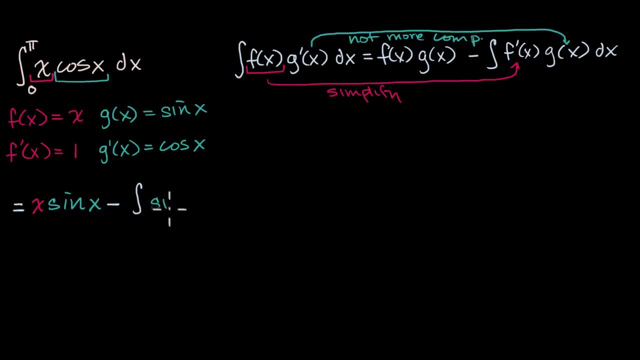 well, we could just rewrite that as sine of x, It'll make it a little bit simpler- Sine of x, dx, dx. And then, remember, this is a definite integral. so we are going to want to evaluate this whole thing. 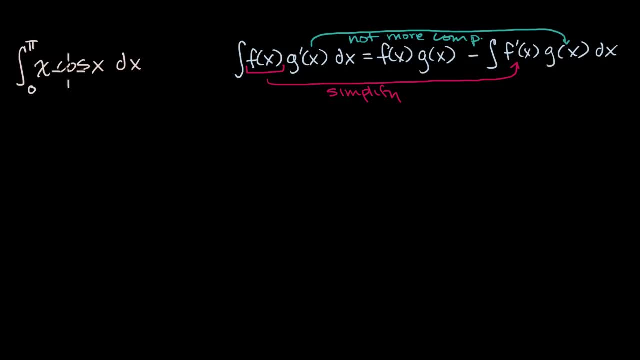 to find the antiderivative of. So let's do that over here: Between x and cosine of x, which one gets more, which one gets more simple when I take its derivative. Well, the derivative of x is just one, So I'm gonna make that my f of x. 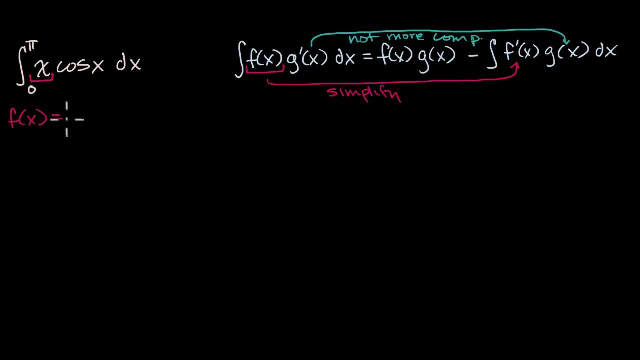 So I could write that over here. So my f of x, I will say, is x, In which case f prime of x, f prime of x, is going to be equal to one. And then what would my g prime of x be? 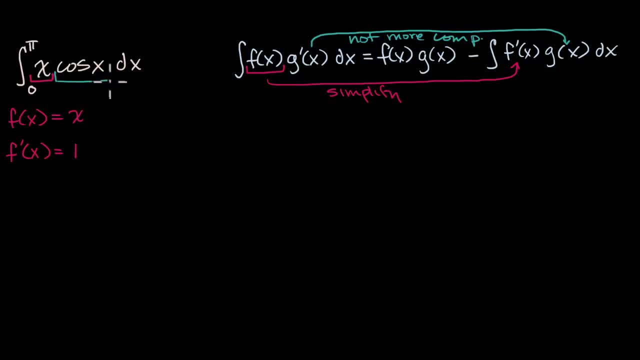 Well, my g prime of x, cosine of x. if I take its antiderivative, it doesn't get more complicated. The antiderivative of cosine of x is sine of x. So let me make that my g prime of x. So g prime of x is equal to cosine of x. 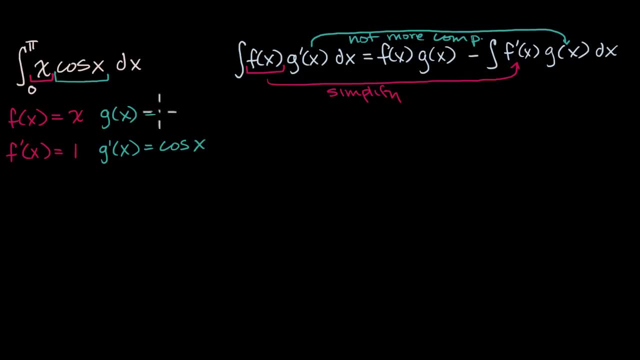 in which case g of x, the antiderivative of cosine of x, well, it's just sine of x, Or the other way to think about it, the derivative of sine of x is cosine of x. Now you could think about plus c's and all of that. 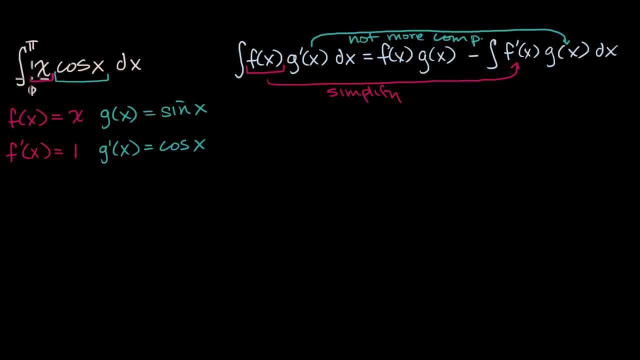 but remember, this is going to be a definite integral, So all of those arbitrary constants are going to get canceled out. So now let's think through this. Let's just apply the integration by parts. Let's just apply the integration by parts here. 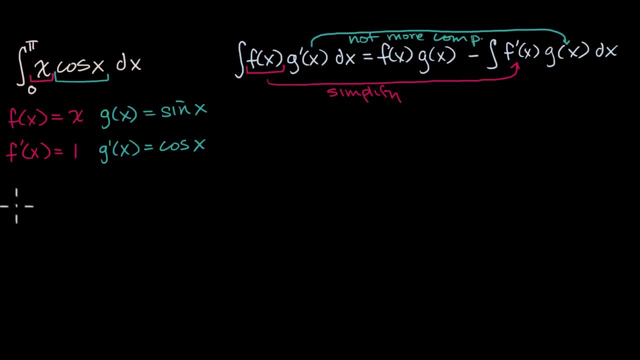 In this particular case, all of this is going to be equal to. so I'm saying that is equal to this. I'm gonna skip down here. It's going to be equal to f of x times g of x. So that is f of x is x, g of x is sine of x. 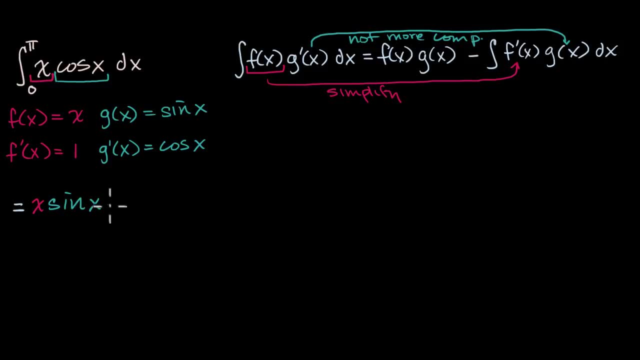 f of x times g of x minus the integral of f prime of x. F prime of x is just one. We could write it like that: one times g of x. g of x is sine of x. So we could write it like this: 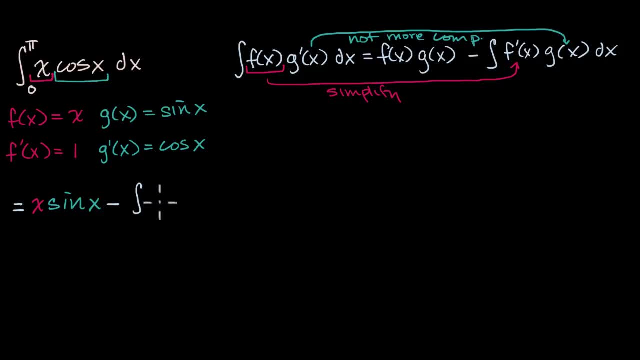 but one times sine of x. well, we could just rewrite that as sine of x, It'll make it a little bit simpler. Sine of x, dx, dx, And then remember, this is a definite integral. So we are going to want to evaluate this whole thing.